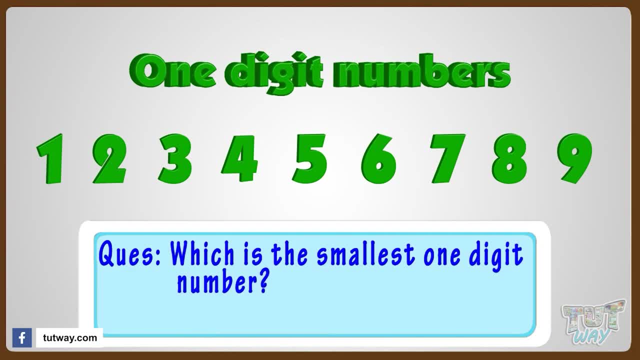 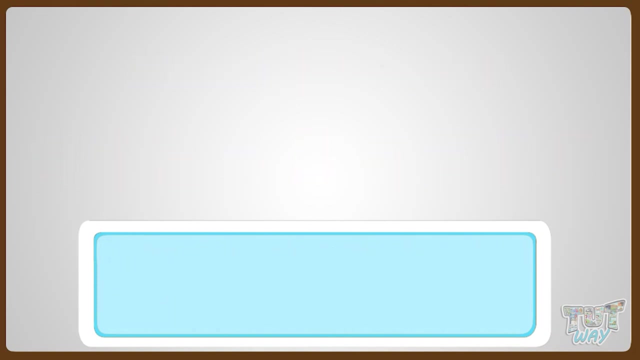 Now which is the smallest one-digit number? One-digit numbers are 1 to 9.. And the smallest number here is 1.. So the smallest one-digit number is 1.. Good, Now which is the biggest two-digit number? Let's find it out. 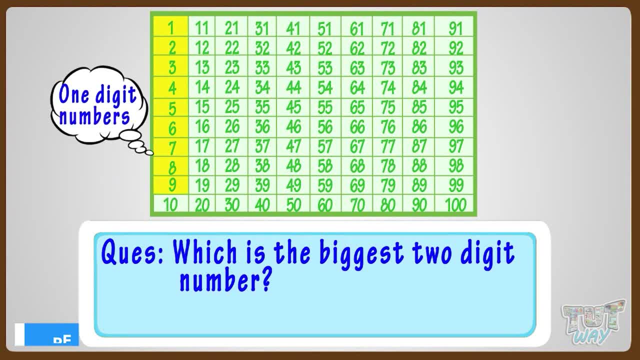 Up to 9, we have one-digit numbers, And from 10 to 99, we have two-digit numbers, As the next number is 100, which is a three-digit number. So 99 is the biggest two-digit number. 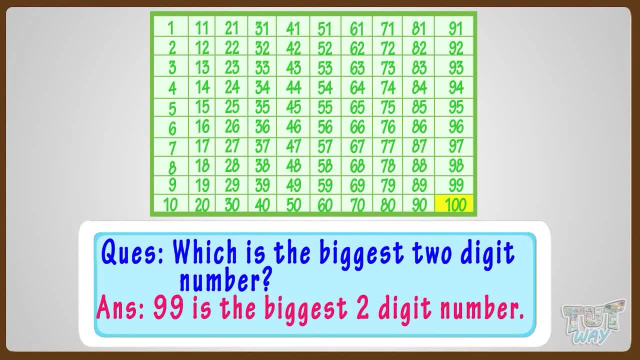 As the next number is 100, which is a three-digit number. Now Let's find out the smallest two-digit number. Can you guess? Okay, two-digit numbers starts from 10.. So 10 is the smallest two-digit number. 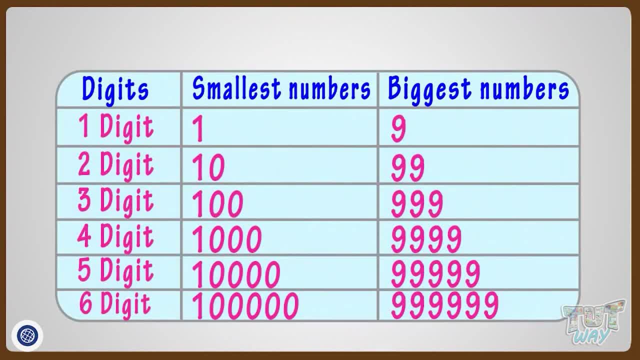 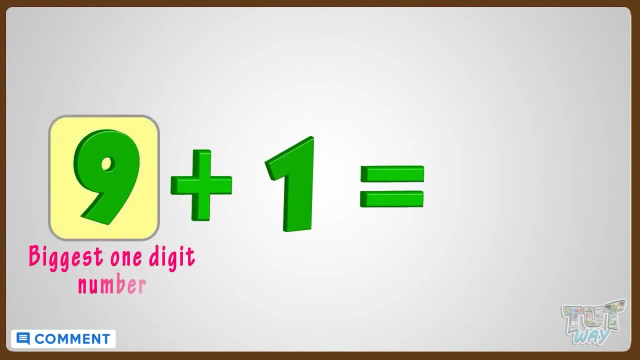 Good. So, kids, here is an interesting pattern to learn Smallest and biggest numbers of particular digits. And the biggest one is 999. And so on. So, kids, if you add 1 to biggest one-digit number, you get the smallest two-digit number. 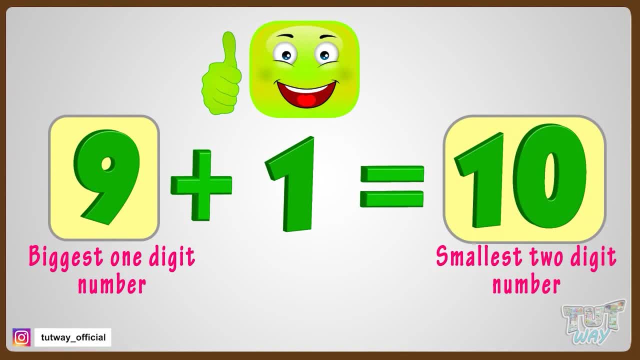 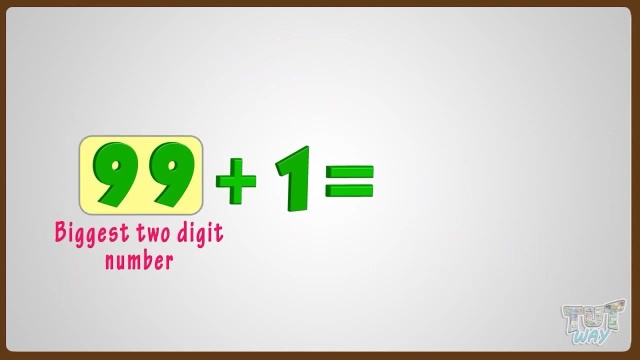 9 plus 1 gives us 10.. And 9 is the biggest one-digit number. Adding 1 to it, we are getting smallest two-digit number. Similarly, if we add 1 to 99,, that is the biggest two-digit number. 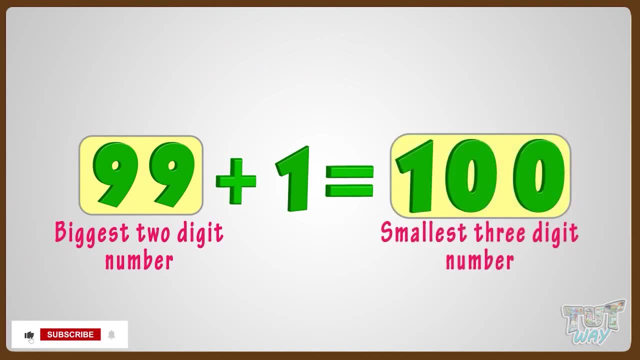 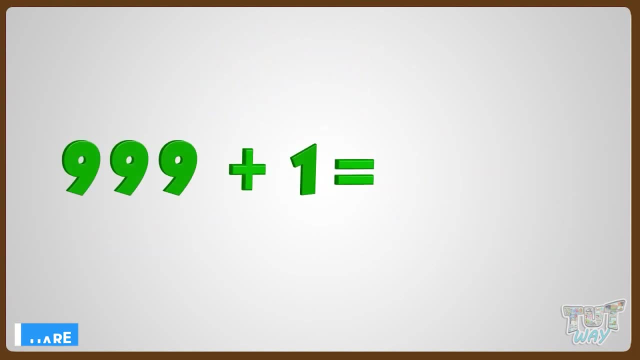 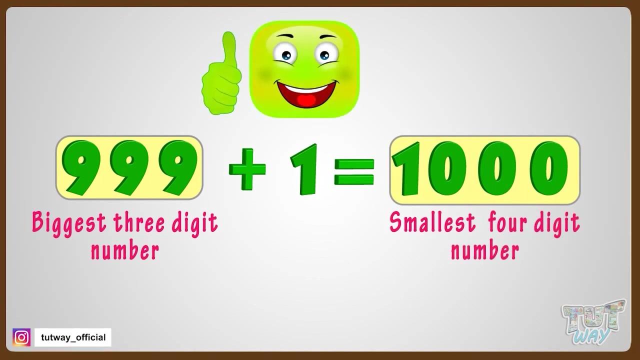 We are getting the smallest three-digit number, that is, 100.. If we add 1 to 999,, which is the biggest three-digit number, we are getting 1000,, which is smallest four-digit number. Now let's learn more. 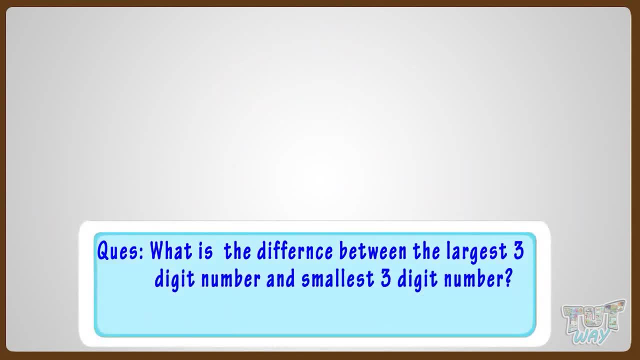 What is the difference between the largest three-digit number and smallest three-digit number? Let's find it out. We are asked to find out the difference. That means we have to subtract the two numbers, And which two numbers? Largest three-digit number, that is 999.. 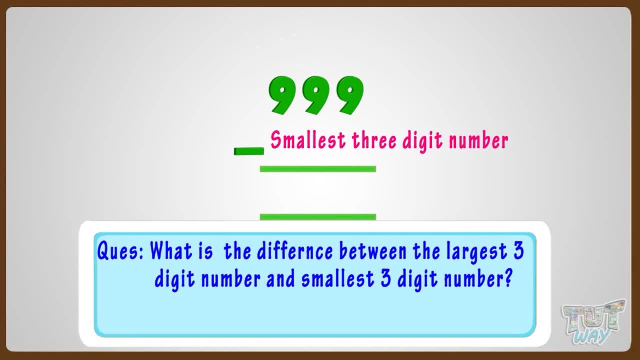 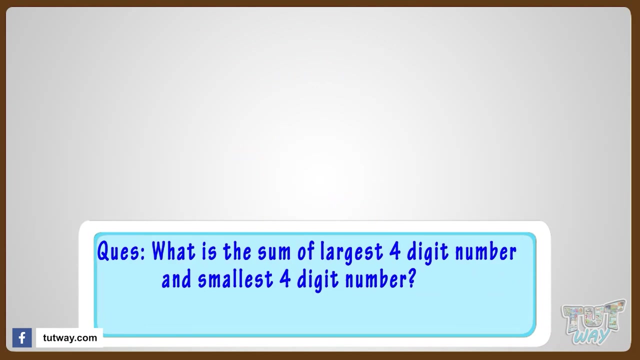 And the smallest three-digit number, that is 100.. So subtract 100.. Subtract 100.. Subtract 100.. From 999, we get 899.. What is the sum of largest four-digit number and smallest four-digit number? Let's find it out. 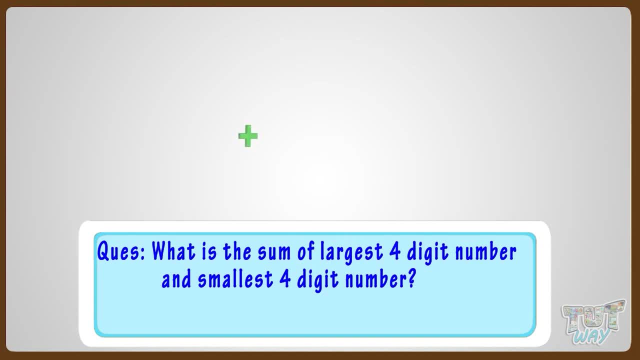 We are asked to find out the sum. That means we have to add the numbers, And which numbers. Largest four-digit number, that is 9999.. And the smallest four-digit number, that is 1000.. So add 9999 and 1000.. 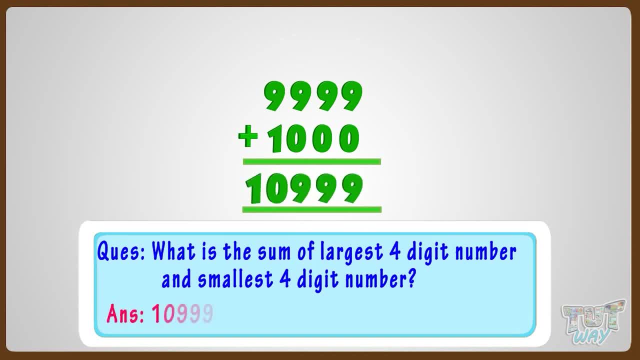 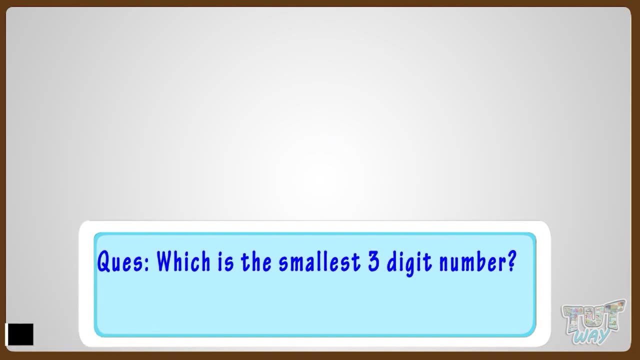 So we get 10,000.. 999. Good, Now let's move to another question: Which is the smallest three-digit number? Let's find it out. Have a look. 1 to 9, we have one-digit numbers. 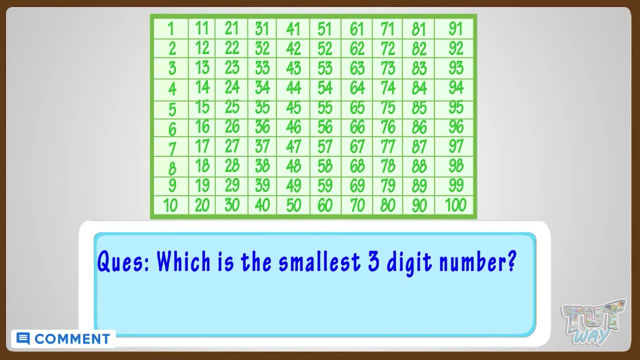 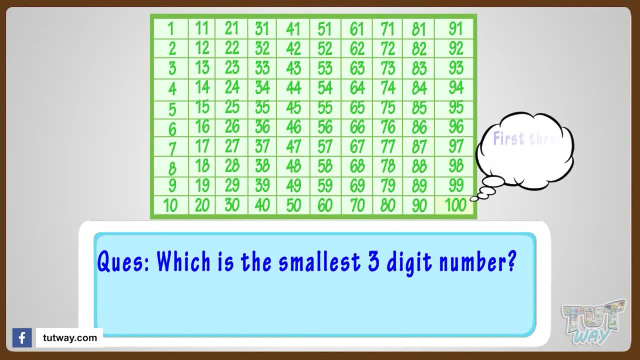 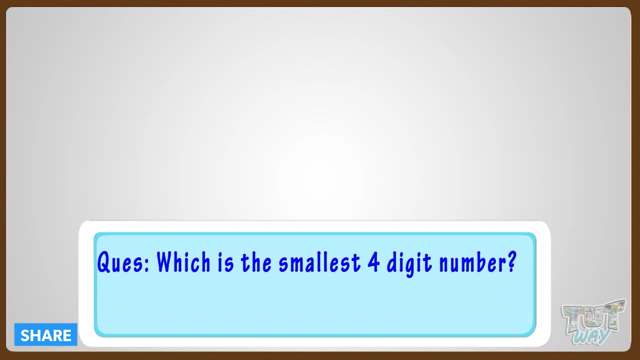 And from 100 starts the three-digit numbers. Hence 100 is the smallest three-digit number, as it is the first three-digit number. Now let's move to the next question: Which is the smallest four-digit number? Let's find it out. 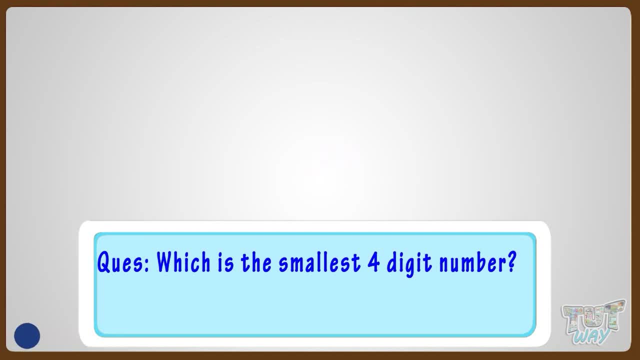 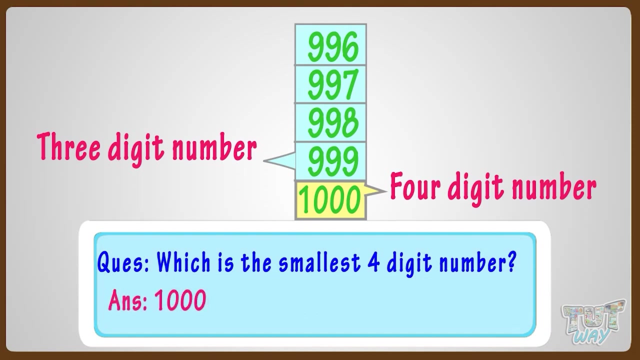 Up to 999, we have three-digit numbers And after 999, we have 1000, which is a four-digit number and the first four-digit number. So 1000 is the smallest four-digit number, Which is the smallest four-digit number. 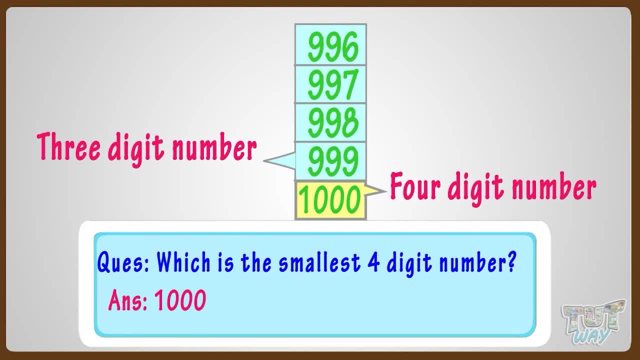 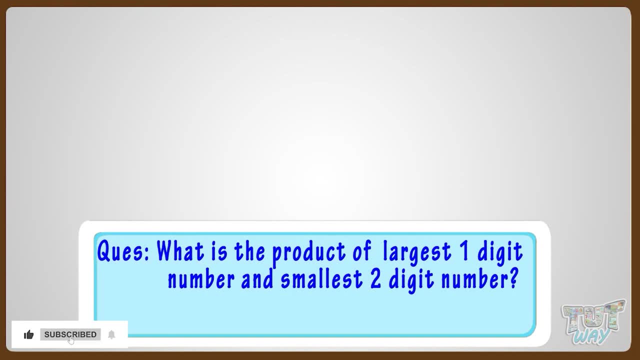 Good, Now let's move to the next question. What is the product of largest one-digit number and smallest two-digit number? Let's find it out. We are asked to find out the product. It means we have to multiply the numbers. 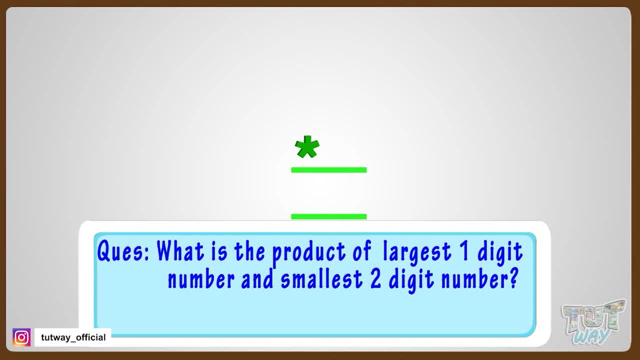 And which numbers The largest one-digit number, that is 9, and the smallest two-digit number, that is 10.. So multiply 9 and 10, and we get 90.. So 90 is the answer Good. 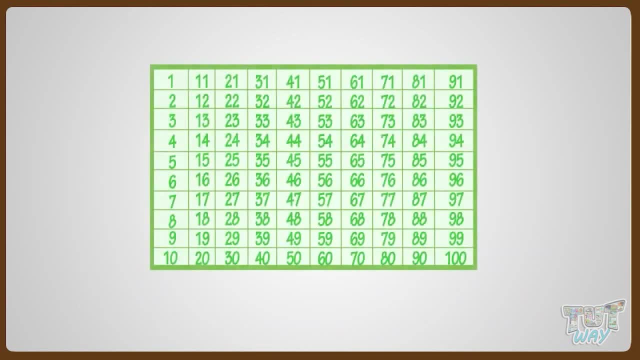 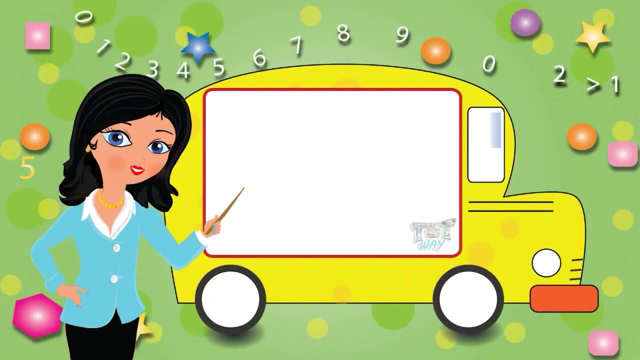 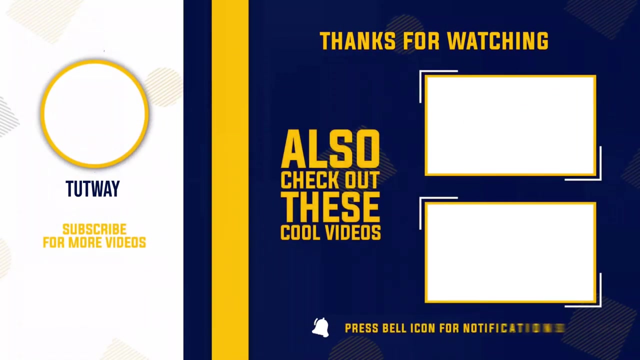 So, kids, today we have learned various smallest and biggest numbers of particular digits. Now you may go ahead and take a quiz to learn more. Bye-bye, Thank you so much for watching. Don't forget to like, comment and share this video. 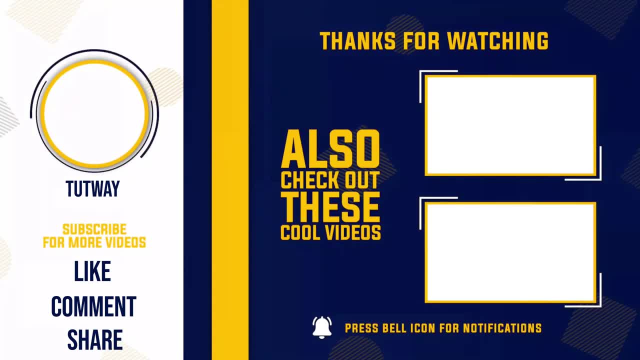 And if you want to see more fun videos, you can hit that subscribe button. You can also follow us on Facebook and Instagram for more content. Bye-bye.